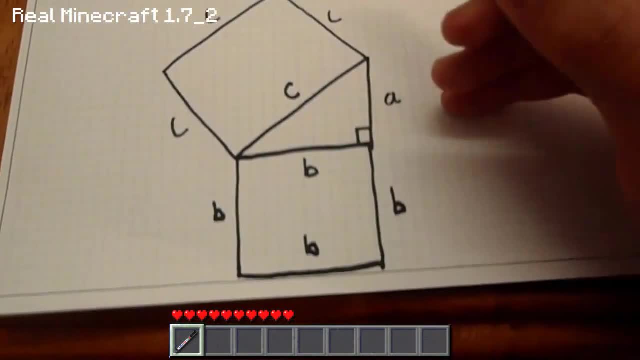 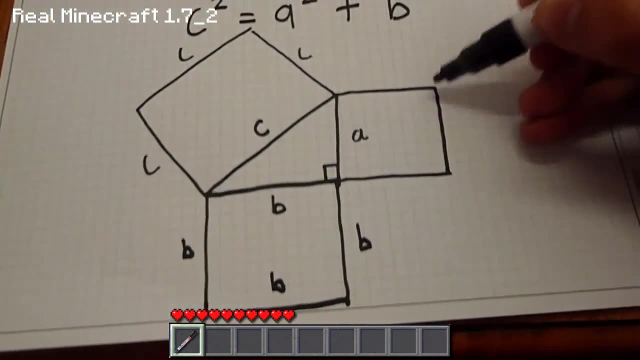 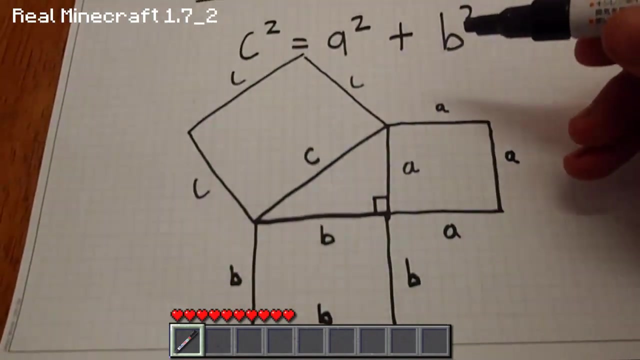 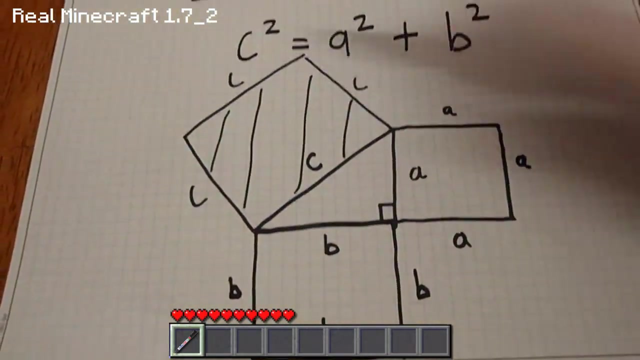 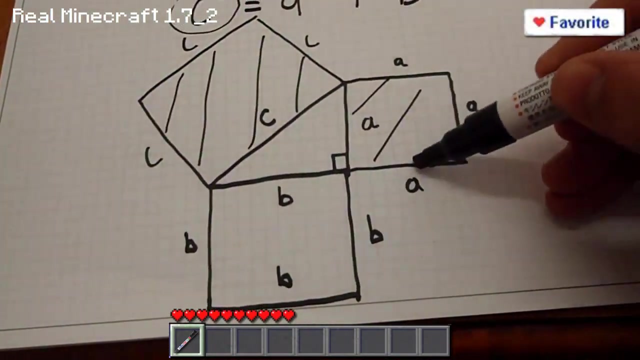 square is B, B and B. so basically it's a square, as I said, and we draw another square off the other side of the triangle so that A, A and A. so basically that square is the same size. What this means is the area of this square here. so C squared equals the area of A plus. 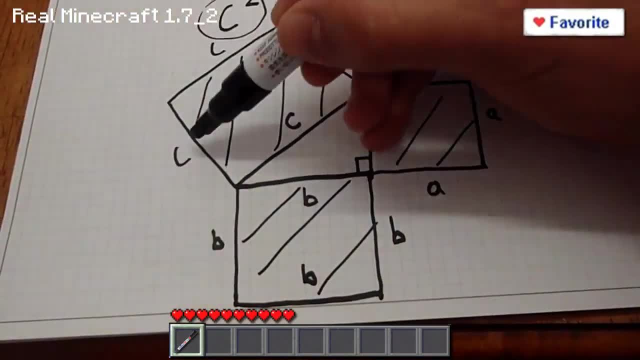 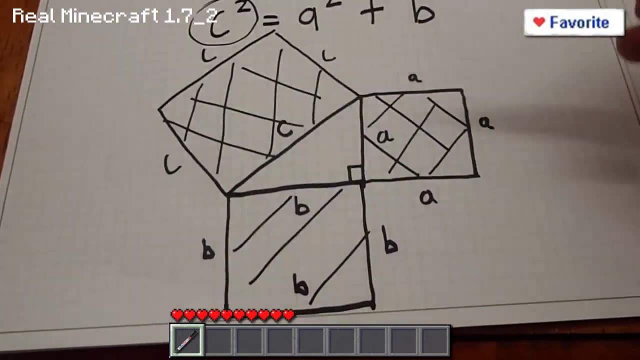 B squared and C squared is C times C, which is the area that I just said, and A squared is the area of here. so A times A is A squared and block wise for B. So basically that's it. basically that's how we proved. 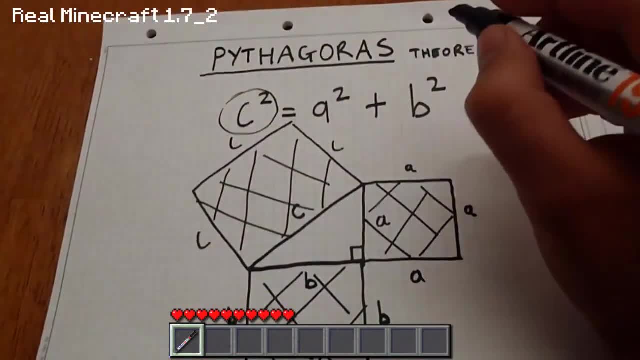 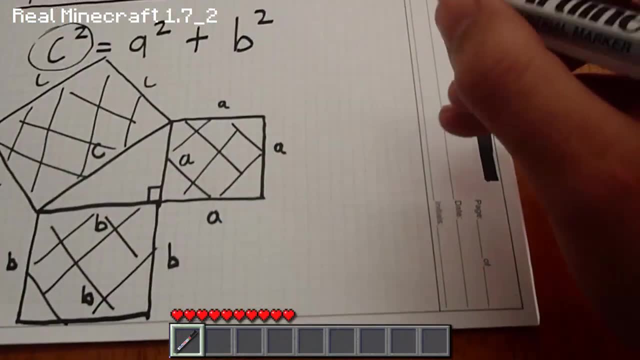 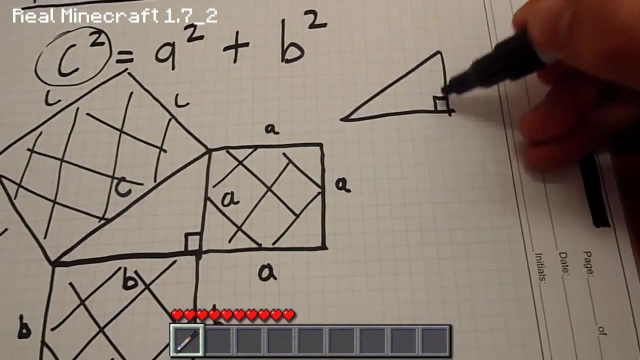 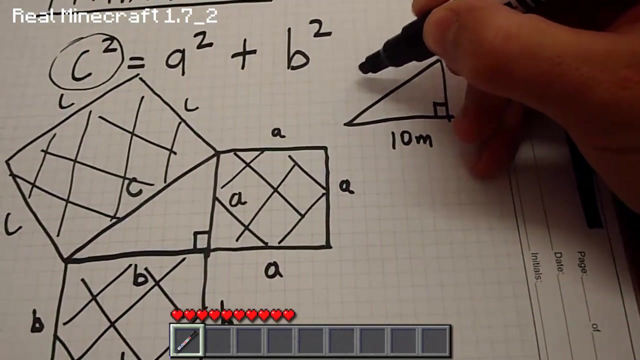 that c squared equals a squared plus b squared. so it's pretty simple stuff. but this can also be used for i'll just draw a quick triangle before we get into the examples. if you have a triangle, say um b is equal to ten meters, um the hypotenuse is equal to just say: 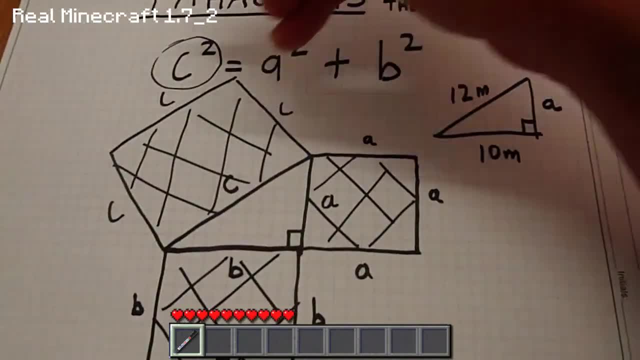 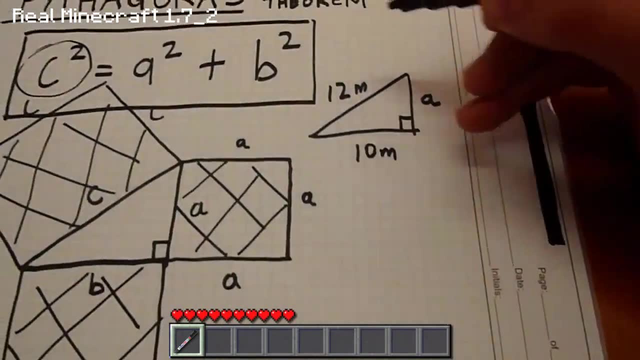 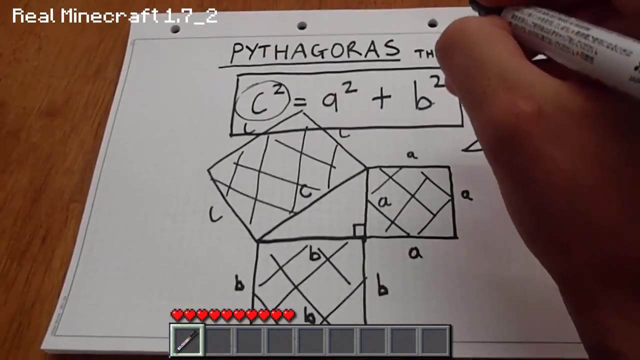 twelve meters. you can actually work out using this equation here the pythagoras theorem, the length of a, and i will go through these examples in a second. but before i go into the examples i want to rearrange this equation so we can get the formulas for c. 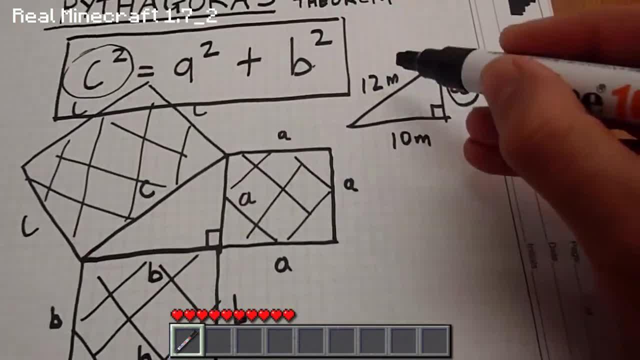 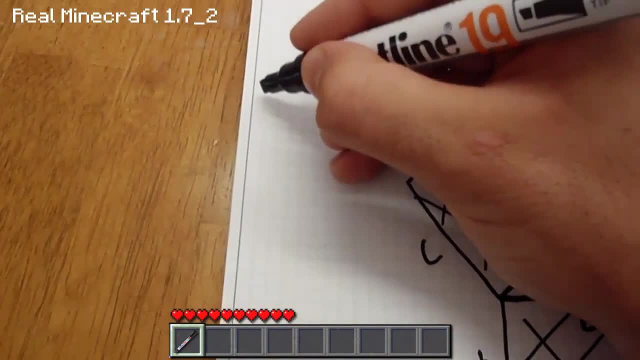 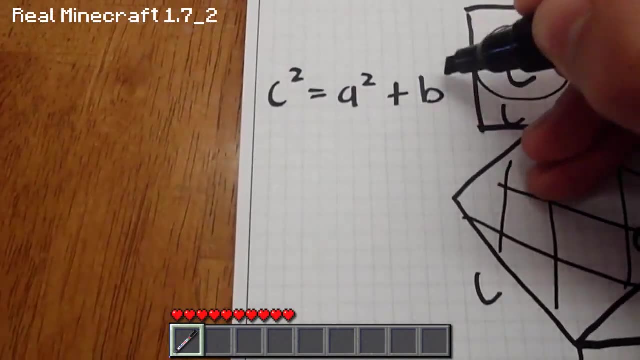 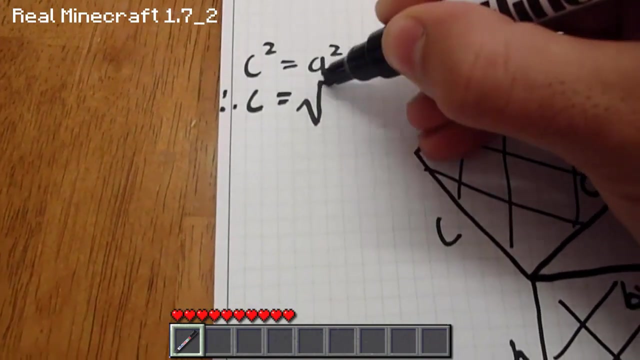 a and b. so if we go to two dimensions of the right handed triangle we can actually work out the missing side. so let's quickly derive that. so first of all, c squared equals a squared plus b squared. therefore, through algebra, c equals the square root. let's do a nice square root sign. 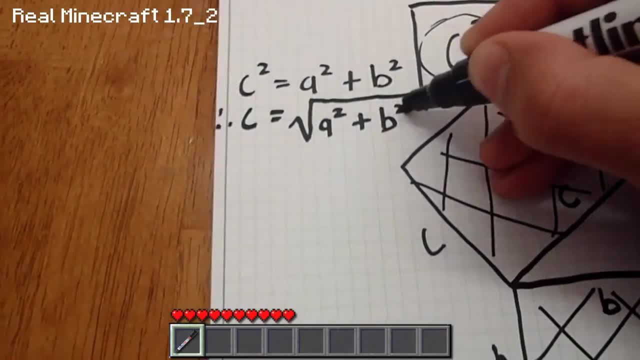 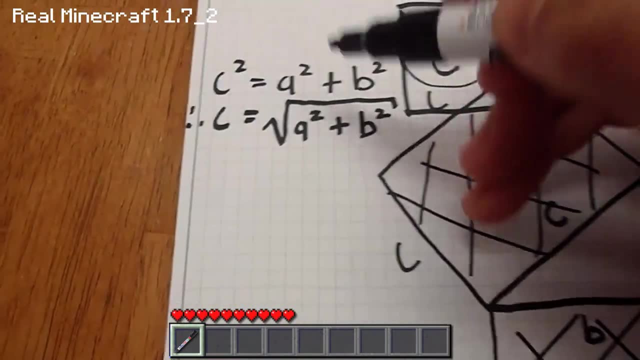 of a squared plus b squared, and that's just simply taking the square root over to the other side of the equal sign basically means you have to square root. and if i were to take my square root over the other side of the equal sign, take the square root over to the other side- I would have the times. That's just basic. 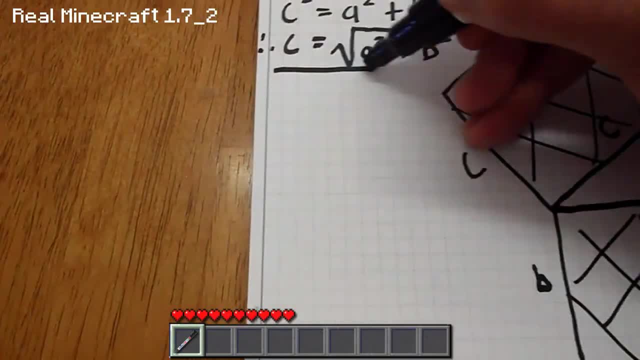 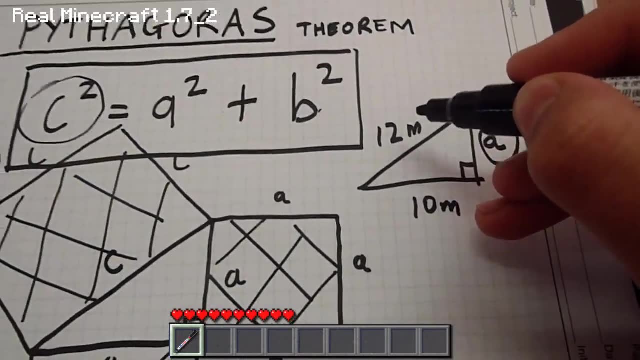 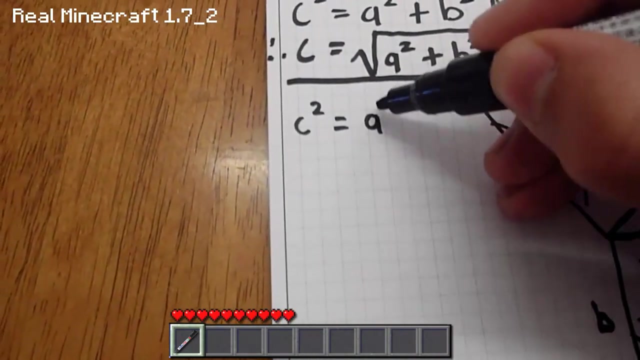 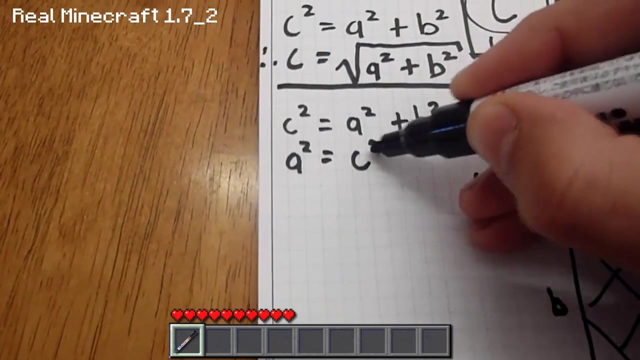 algebra. So let's just look into. so that's the equation for C. So if I know A and B over here I can work out what the hypotenuse of the triangle is. So let's just work out this for A now. So C squared equals A squared plus B squared. Therefore A squared equals C squared. 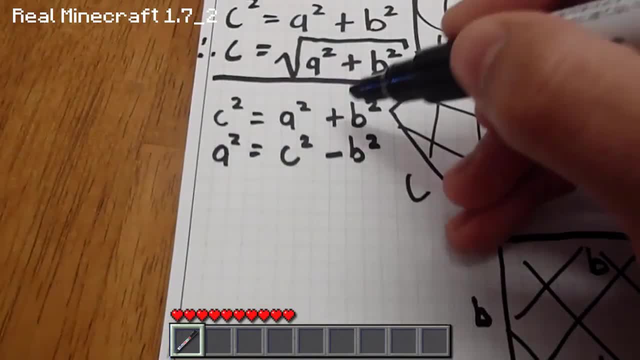 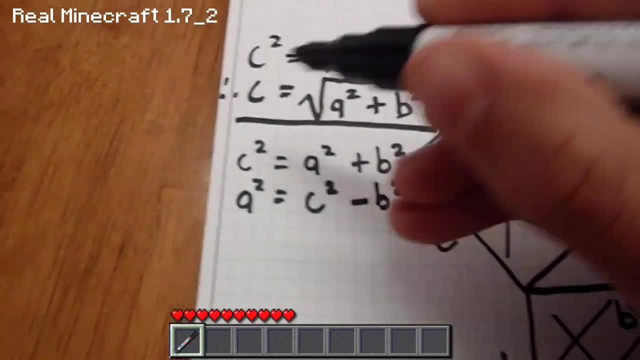 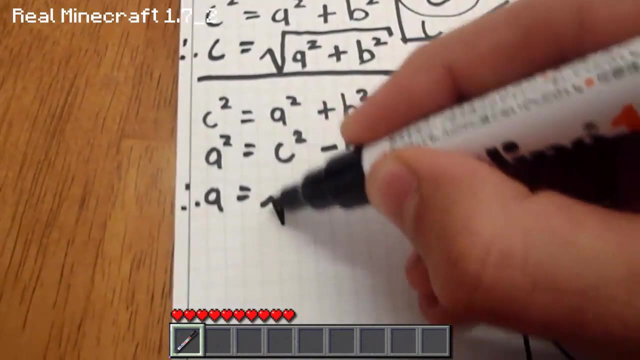 minus B squared. Now what I did there was all I did was I just took B over to the other side and because it's plus B, I have to minus it over the other side. So A squared equals C squared minus B squared. Therefore, A equals the square root of C squared minus B squared. 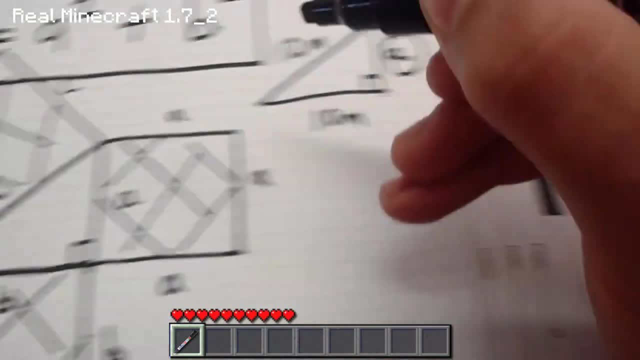 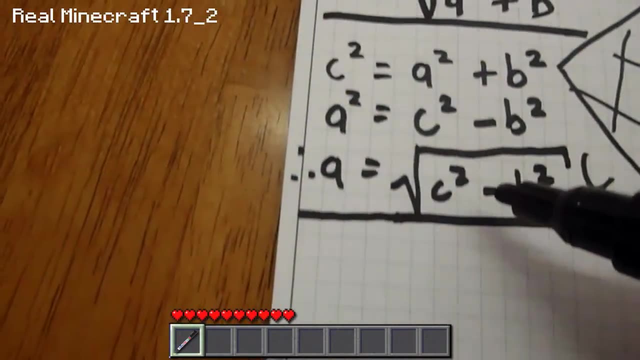 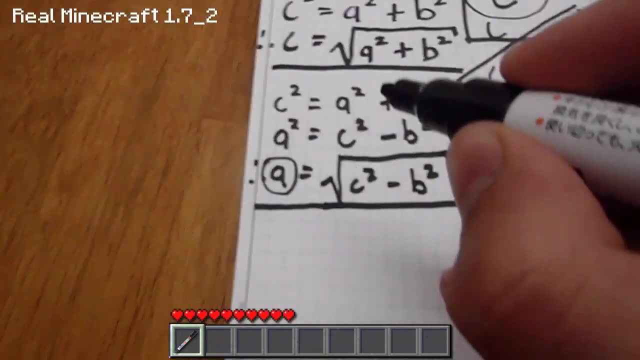 which is So. therefore, if I chuck 12 into what's over here into C, and if I chuck 10 into B, I could theoretically work out what A is in this right-handed triangle And without deriving B. I'll simply just write it down here- And B, if you do. 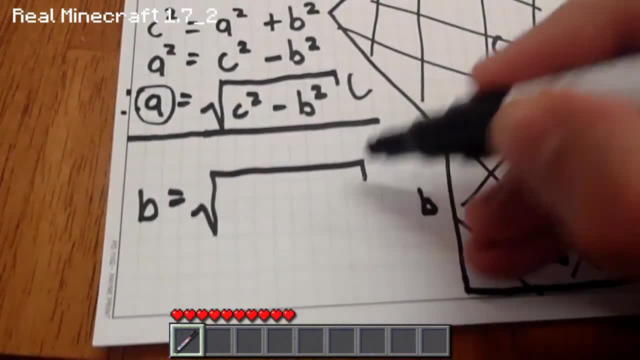 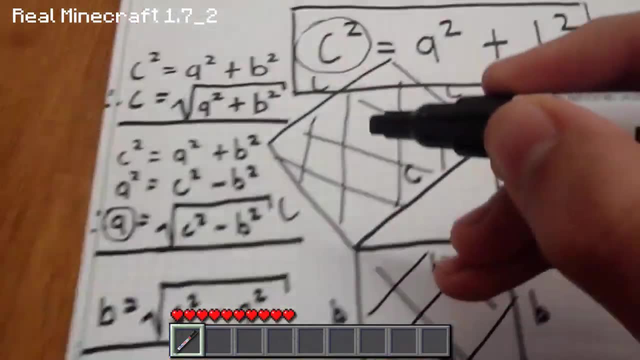 the same thing as I did before, same procedure. you'll get: B equals the square root of C squared minus A squared. So there are your basic formulas from the hypotenuse- sorry, hypotenuse- from the Pythagoras theorem. 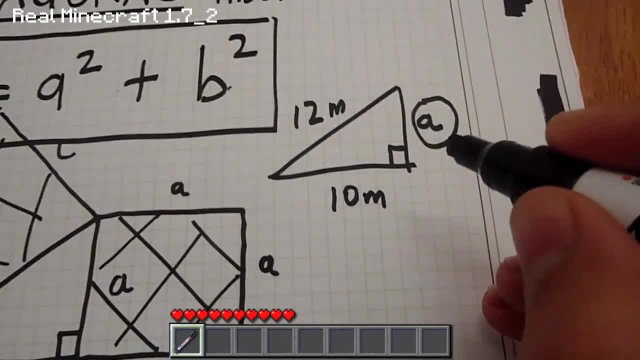 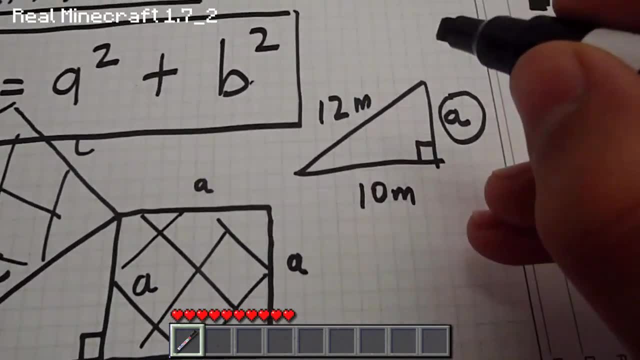 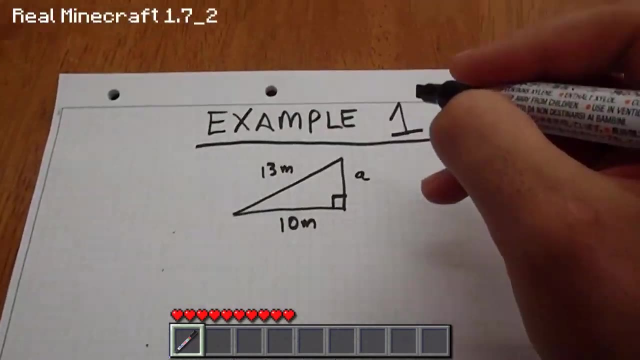 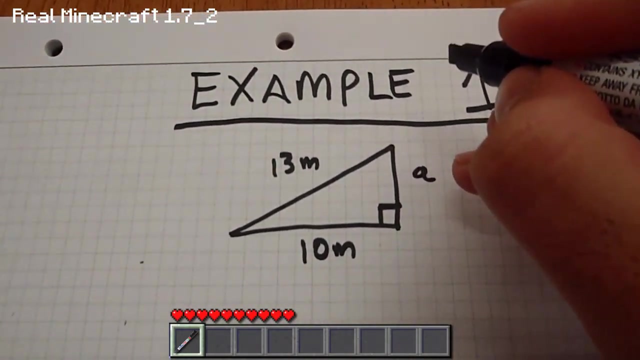 So let's look at some examples now. So let's look at example 1.. We have a right-hand, we have a right-angled triangle with the hypotenuse being 13 meters, the B being 10 meters and the unknown length being 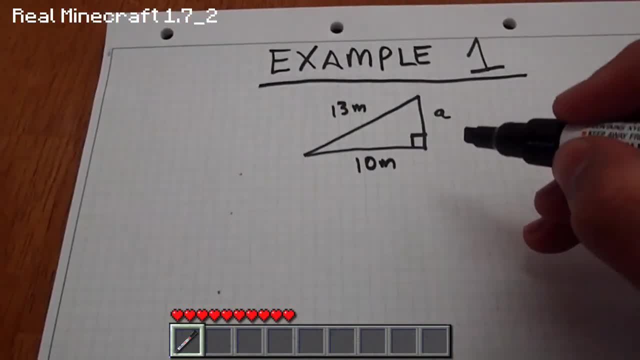 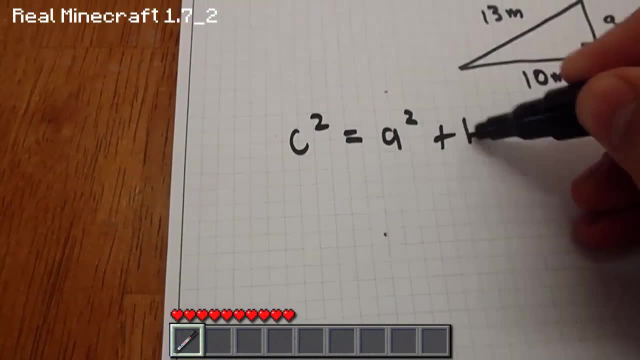 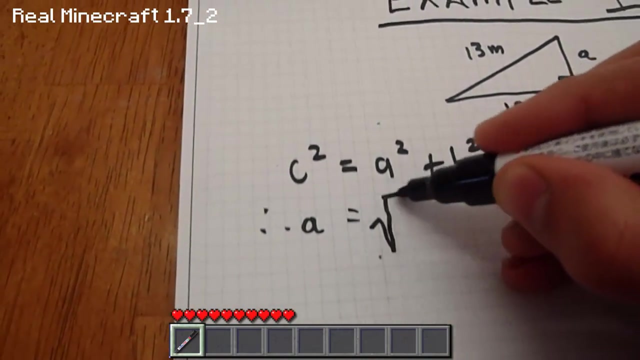 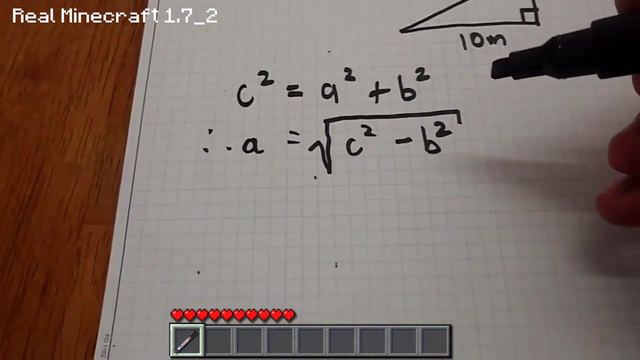 8 meters. So from the equation before, let's describe it quickly again: C squared equals A squared plus B squared and with rearranging that therefore, A equals the square root of C squared minus B squared. So if you throw these, 13 is C, because it's the hypotenuse. 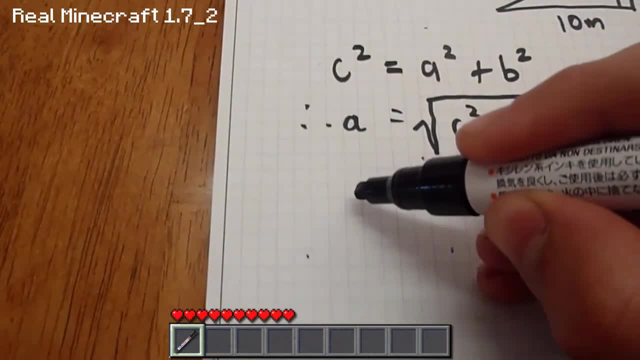 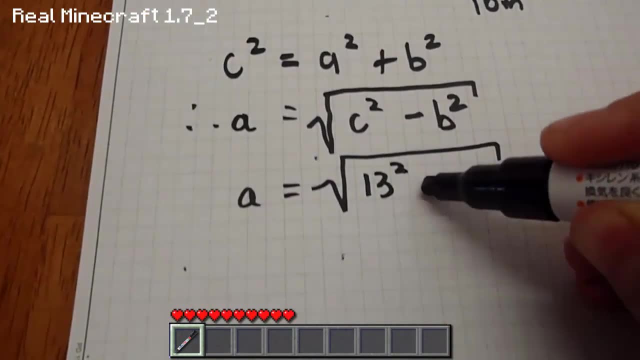 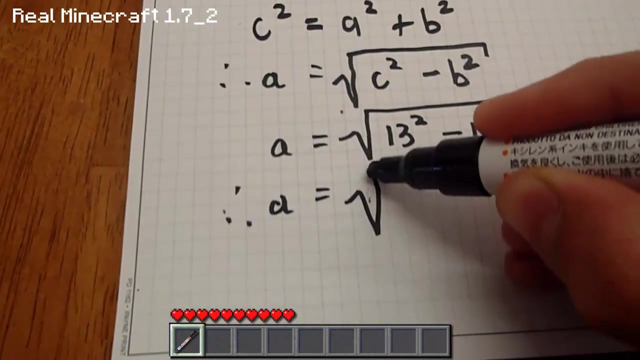 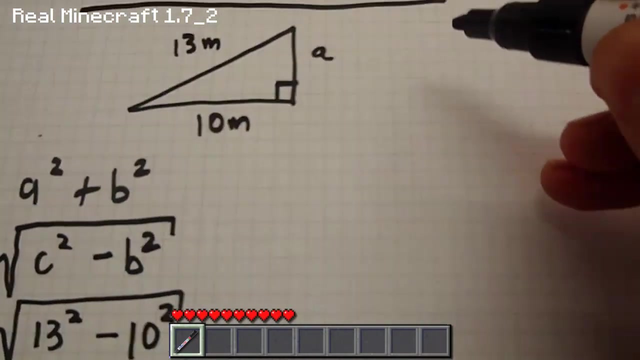 B is 10.. If we throw those values into the equation, therefore, A equals the square root of 13 squared minus 10 squared. Therefore, A equals the square root of 169 minus 100.. Let's go up over here. 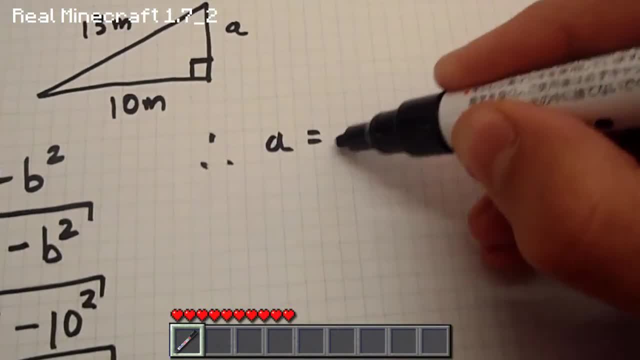 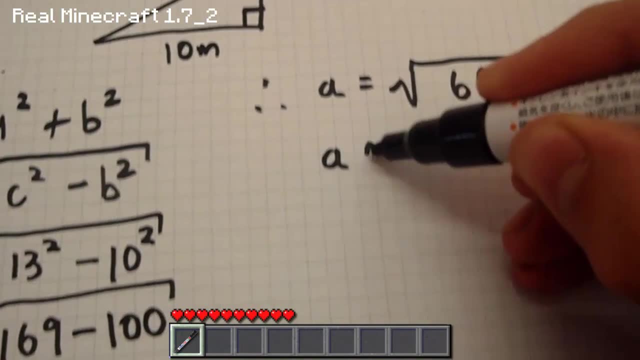 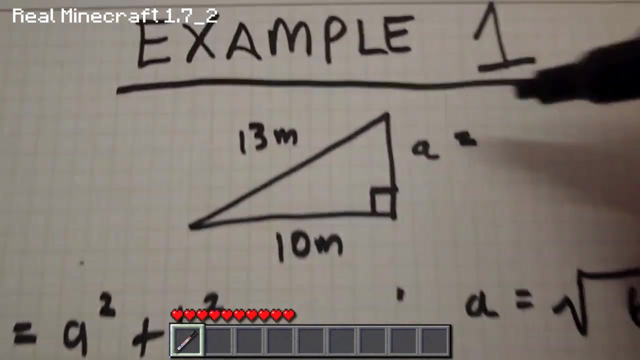 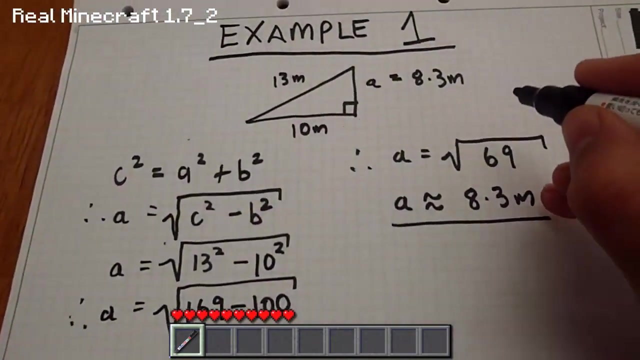 Therefore, A equals the square root of 69, which is A approximately equals 8.3 meters. So the length of A equals 8.3 meters. Pretty simple stuff, And that is using the Pythagoras theorem to work out the distance of. 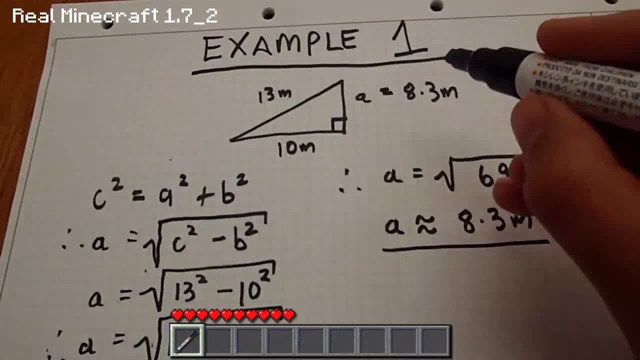 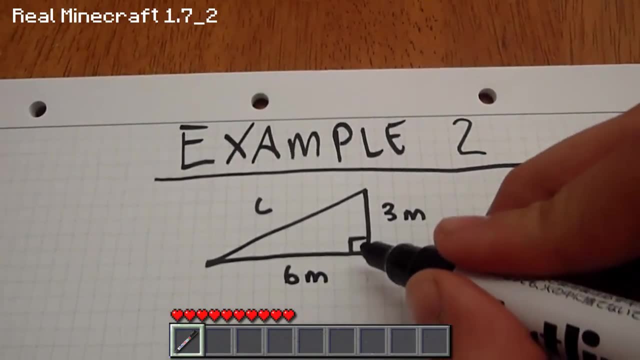 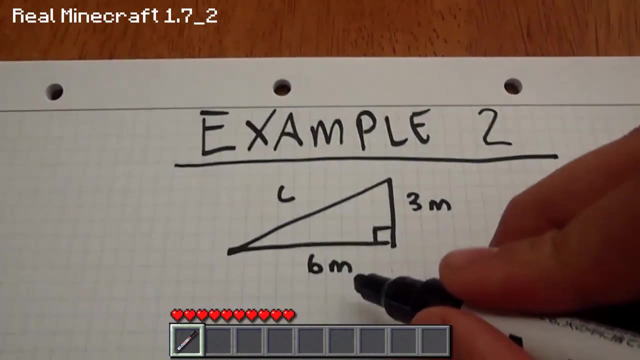 a side of a triangle when you know the other two sides. So let's get into another example now. So let's get stuck into example number two, where we know that this right-handed triangle has one side 3 meters, one side 6 meters, and we don't know the hypotenuse of the triangle. 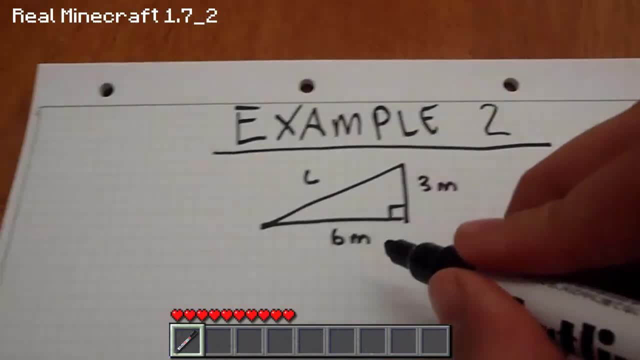 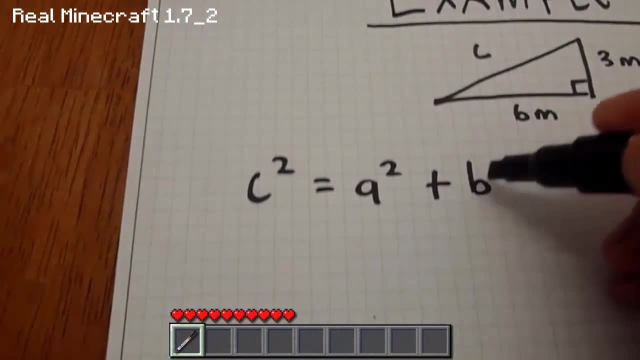 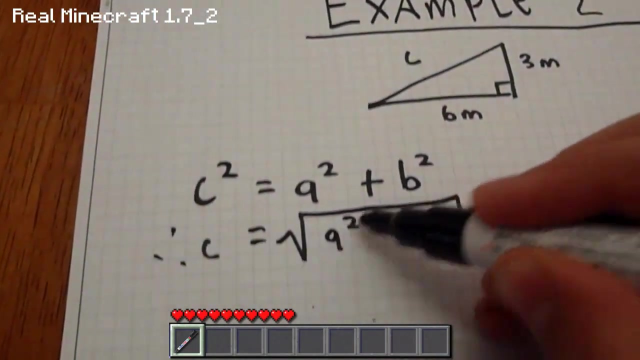 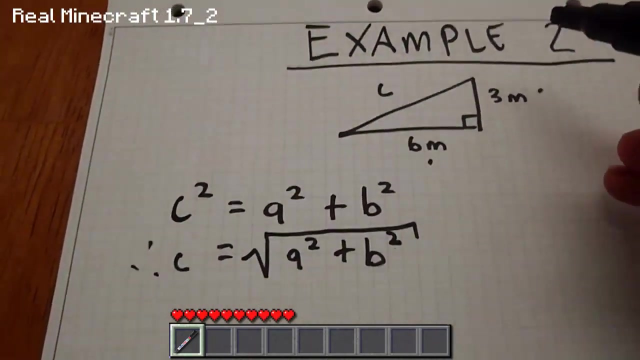 So we can work this out using the Pythagoras' theorem. So, once again, C squared equals A squared plus B squared. Therefore, C equals the square root of A squared plus B squared. Now we know what A is and we know what B is, because they're already stated in the problem. 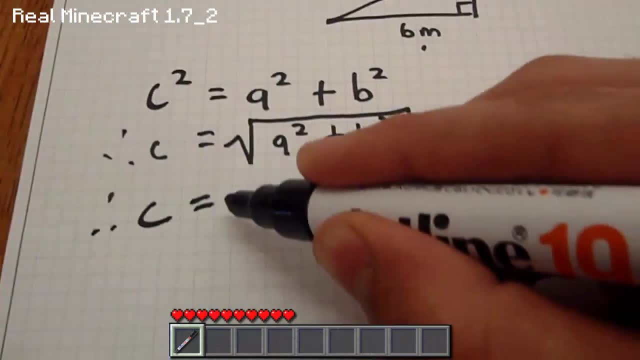 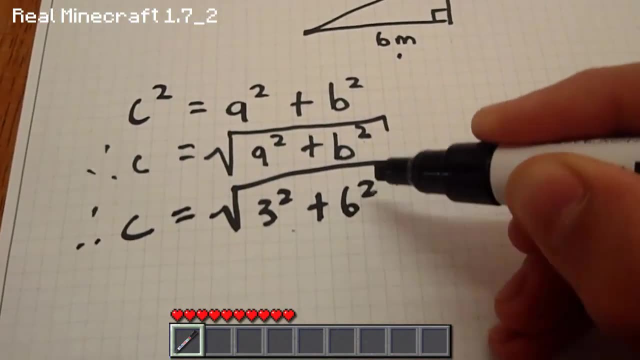 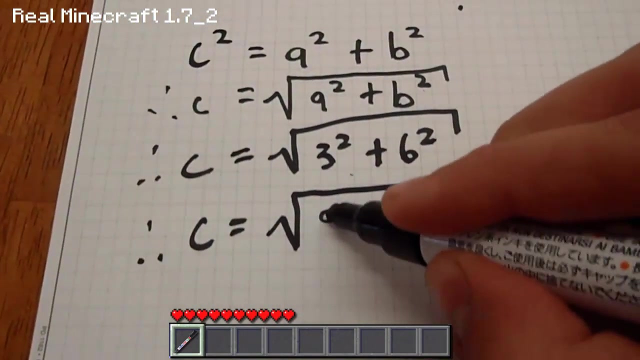 Therefore, C equals the square root of 3 squared plus 6 squared. Therefore, C equals the square root of 9 plus 36.. Let's go over to the right-hand side here, because we've got no room in the bottom. 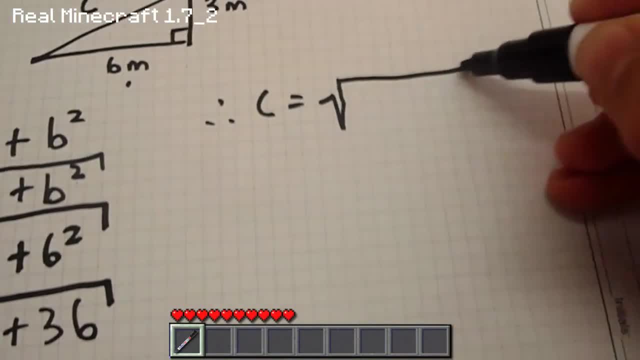 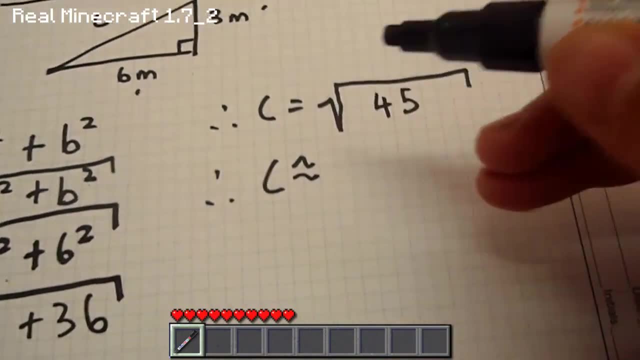 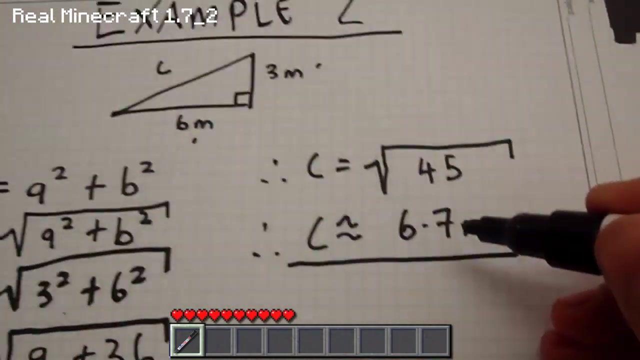 Therefore, C equals the square root of 45.. Therefore, C approximately equals 6.7 meters, Without going into too much detail because that decimal point carries on to about 17,000.. No, I'm just joking About 100..